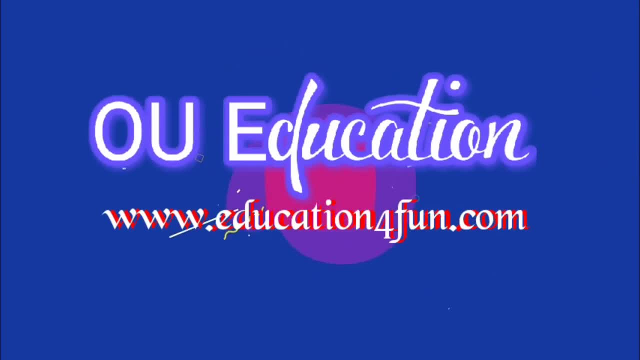 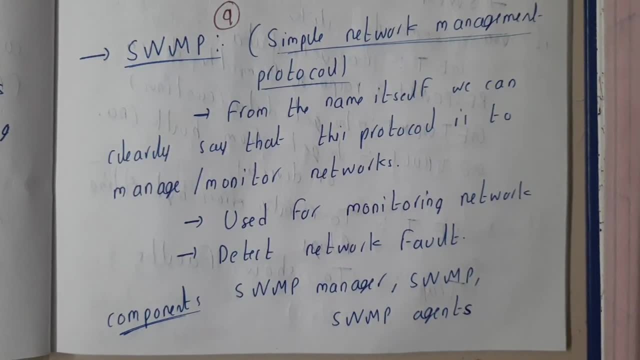 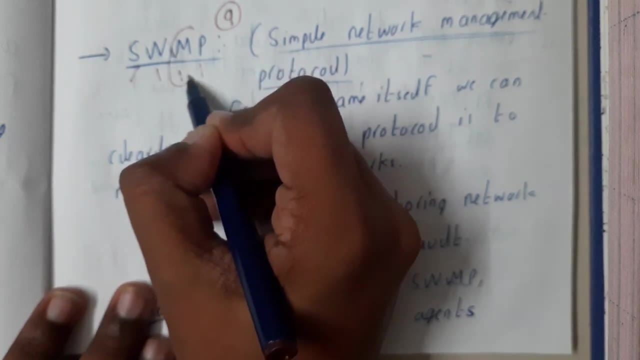 Hello guys, we are back with our next lecture. In this lecture let us go through SNMP. It is nothing but a simple network management protocol. So from this word only you will be saying like it is not a common type of protocol, It is a management protocol. It is used to do management. 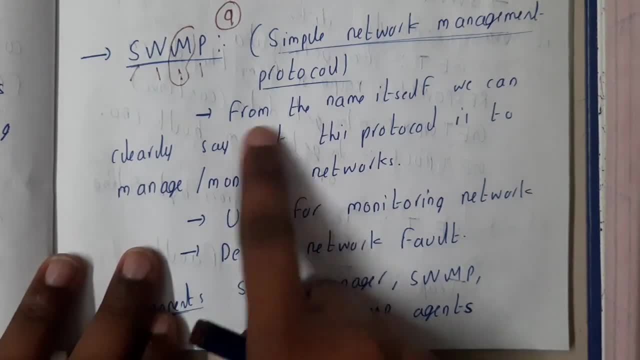 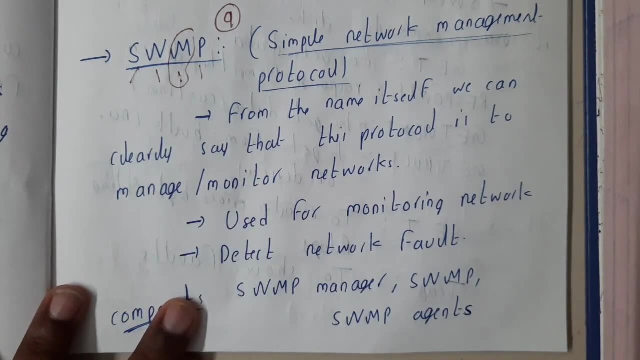 of multiple things or monitoring multiple things, right? Yes, So from the name itself we can clearly say that this protocol is meant for management or monitoring the network. Yes, So used for monitoring the network, detecting any network failures. we will be using this, guys. 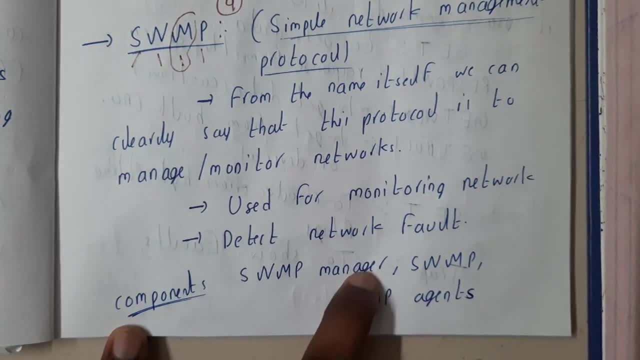 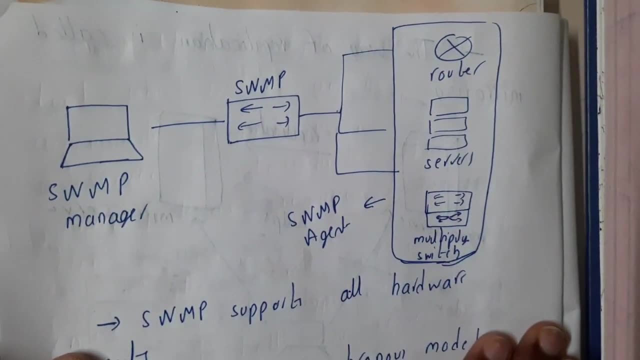 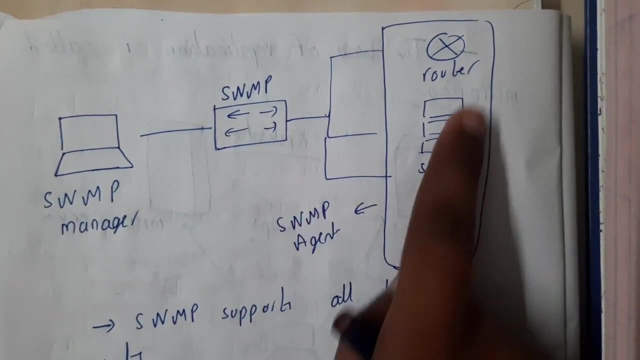 So the components used here are nothing but SNMP manager, SNMP agent and SNMP. Okay, Okay. So if you draw a small diagram, it will be in this way, guys. So the SNMP manager will be connected to the SNMP and this SNMP is connected to the agent. Agent is nothing. 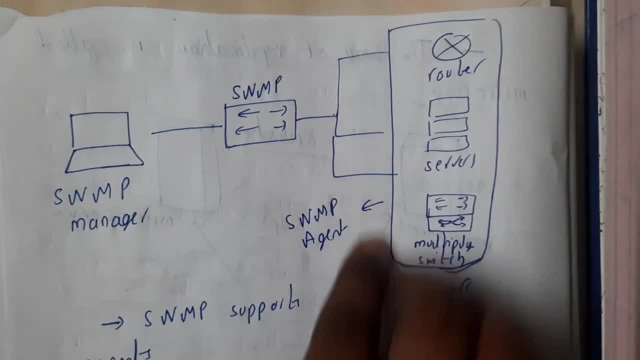 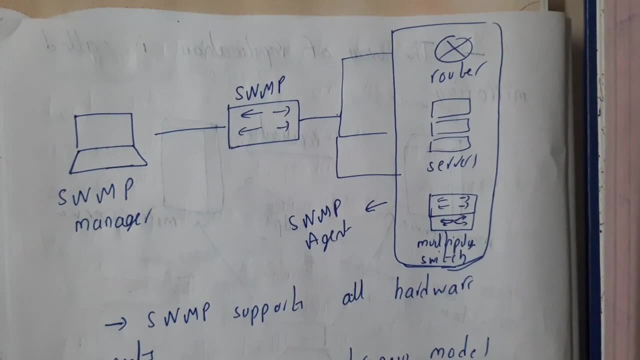 but collection of multiple things guys- routers, servers, switches and all those things will be calling it as combined, We can call agent and he will be observing all these things as statuses like whether they are working and all those things. Okay, So SNMP supports on all hardware. 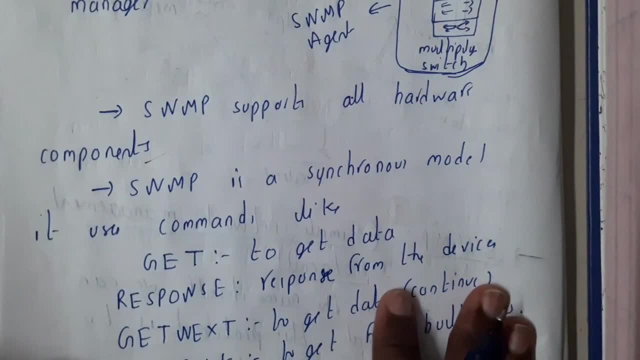 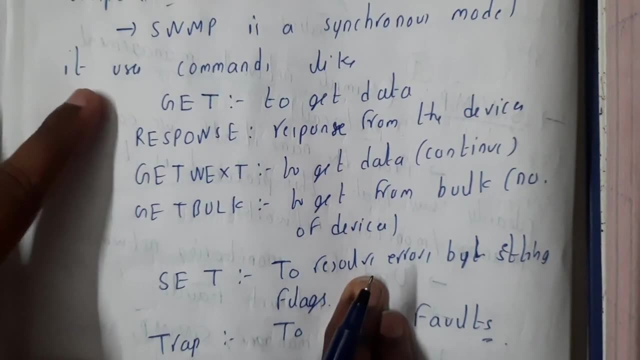 components, guys. That's one of the advantage, Okay. Similarly, SNMP is a synchronous module, guys. Okay. So it's a command. It's commands are as usual as HTTP only. So get is there to get the data Response is there to respond. So it's a command. It's a command. It's a command, It's a. 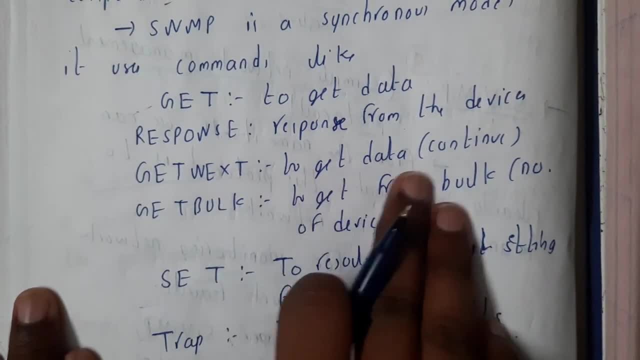 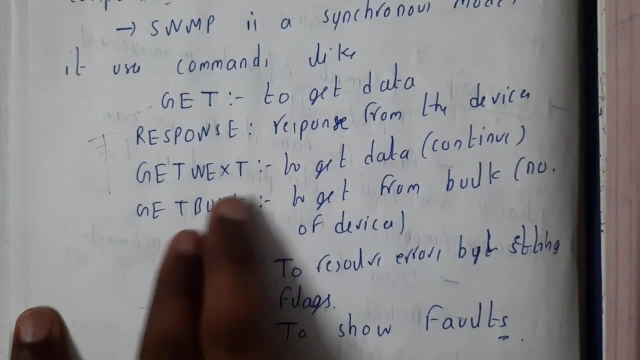 response from the device. Okay. So get next is to get data continuously, like until the end of the information, Like if there are a hundred systems to get to one after the other. we'll be using this. get next, guys. Okay. Similarly, get bulk is to get from a number of devices. So 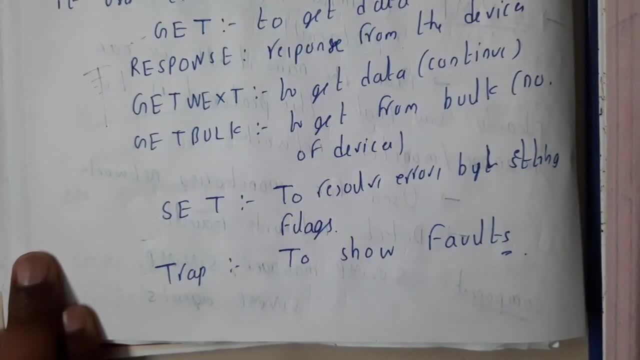 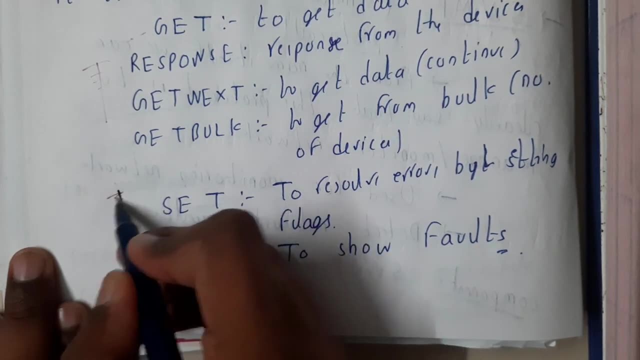 one to 10,, 10 to 20, like that. Okay, Set is used to resolve error by setting the flags and all those things. So assume that there is a flag. due to some error, it became one, So you resolved it. 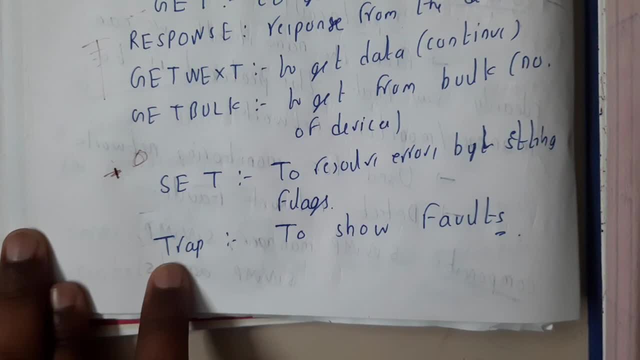 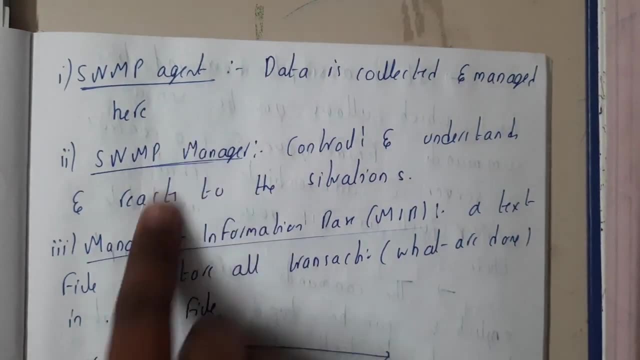 So you need to update it right. So in that situation, you'll be going for set. Similarly, trap is nothing but to show any kind of faults. You'll be entering those flags and all those things, Okay, Okay. So now let us go.